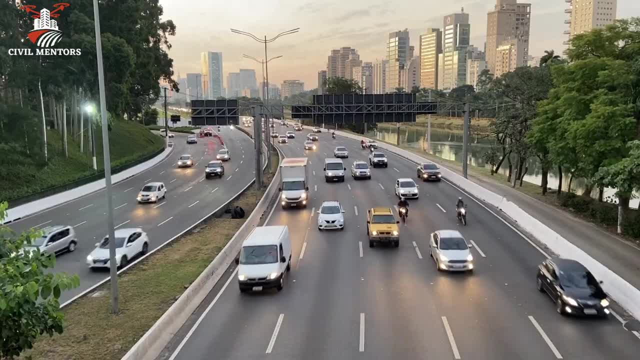 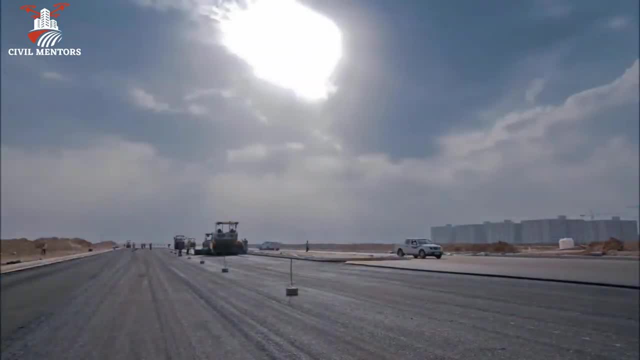 Every day, millions of people rely on roads to commute, to work, transport goods and travel to new destinations. But have you ever wondered how these roads are constructed and what goes into making them safe and durable? Roads are the lifeline of any society, and modern road 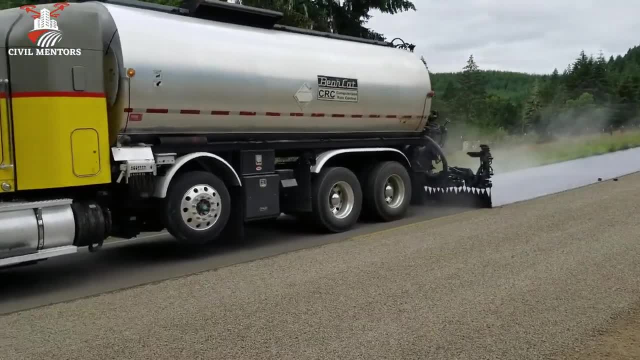 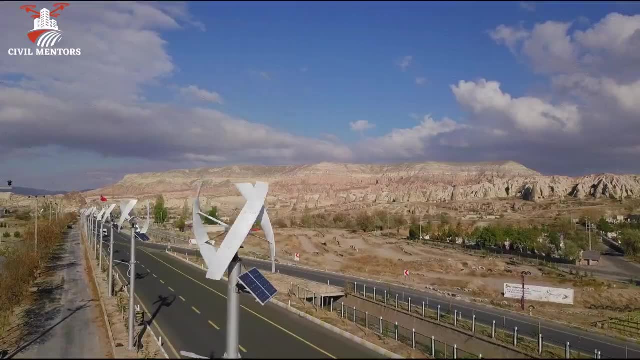 construction techniques have transformed the way we build and maintain them. From highways to small streets, the process of road construction has evolved over the years to become more efficient, eco-friendly and durable. In this video, we will take a closer look at the step-by-step. 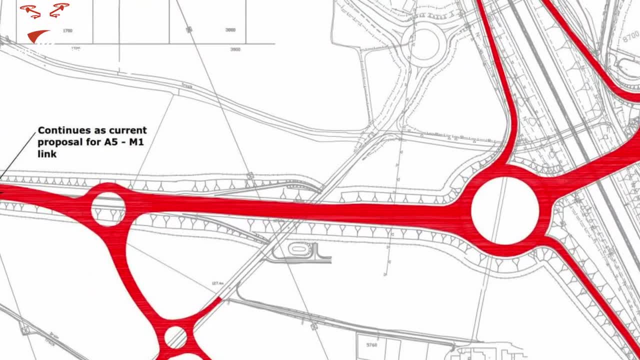 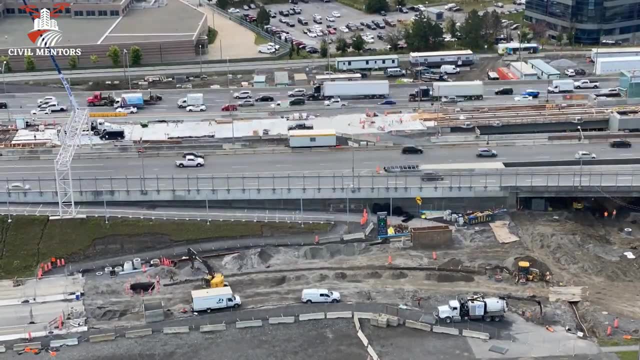 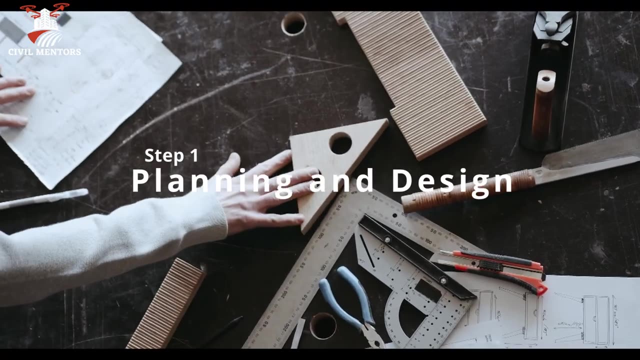 process of road and highways construction, from planning and design to opening up to the public. We'll explore the latest engineering techniques and equipment used to construct durable and sustainable infrastructure that meets the needs of our communities. The first stage in modern road construction is planning and design. 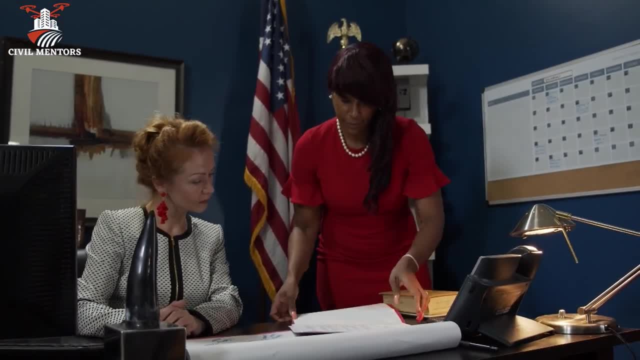 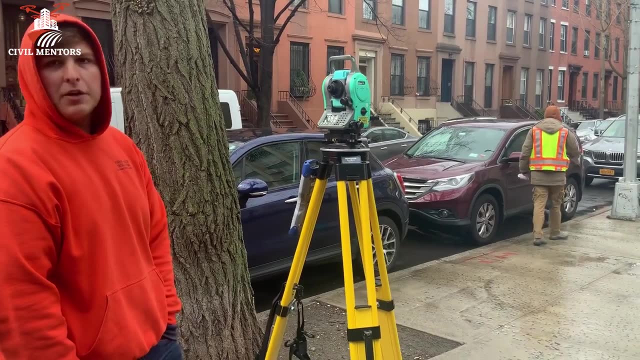 During this stage, engineering and construction techniques are used to build and maintain roads and highways. The first stage in modern road construction is planning and design. During this stage, engineers work closely with local authorities to assess the road's purpose, expected traffic volume and environmental impact. They also conduct surveys to determine the site's topography. 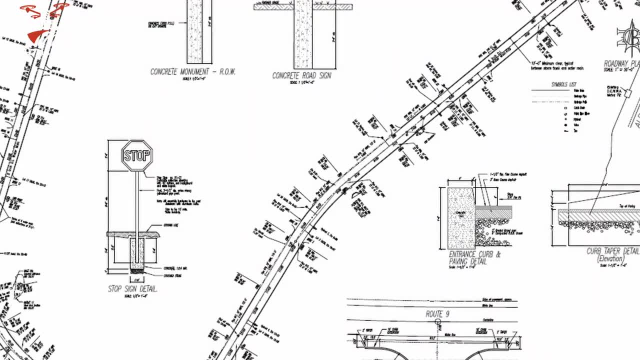 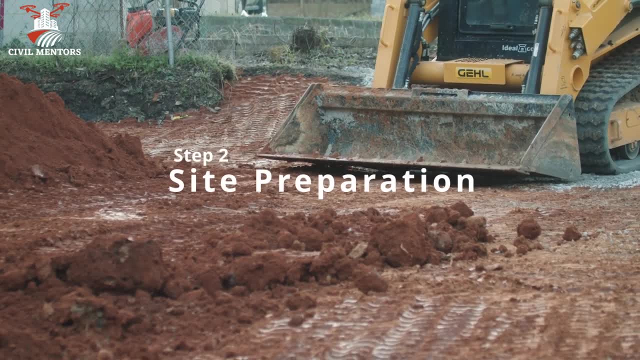 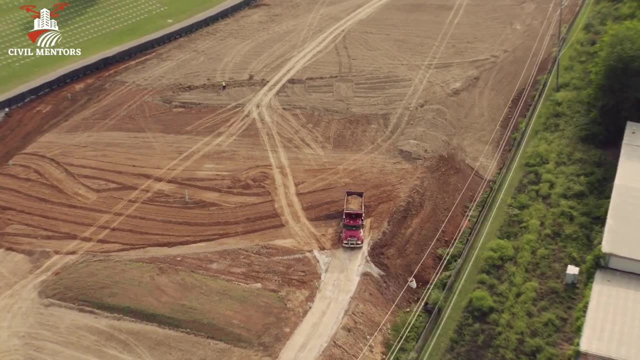 and soil conditions. Based on this information, engineers create a detailed design plan that includes the road's alignment, cross-section and drainage system. Once the planning and design stage is complete, the next step is to prepare the site for construction. This may involve clearing trees. 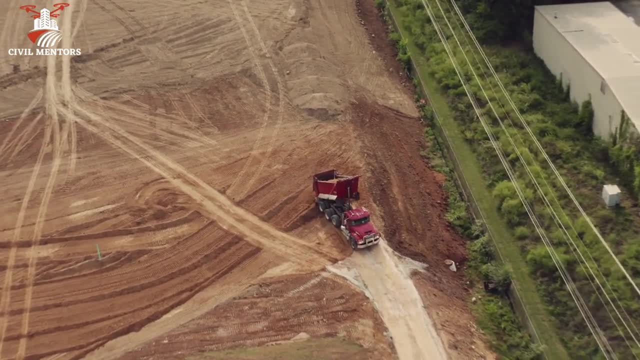 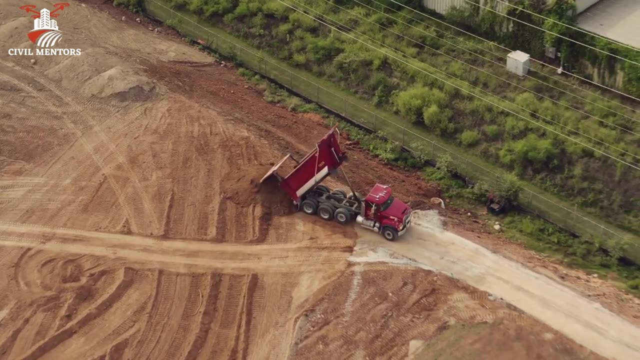 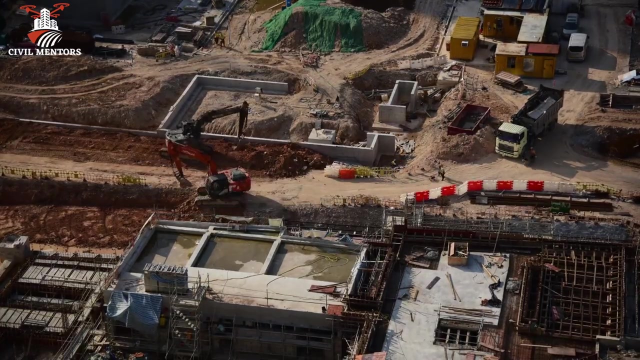 and other vegetation, removing existing structures and grading the land to create a level surface. The soil may also need to be stabilized to prevent erosion and provide a strong foundation for the road. With the site prepared, it's time to start building the road's foundation. 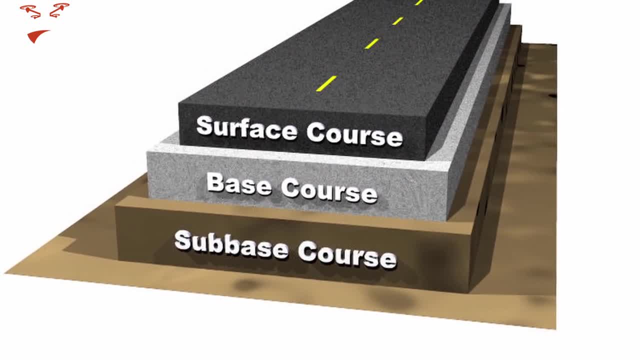 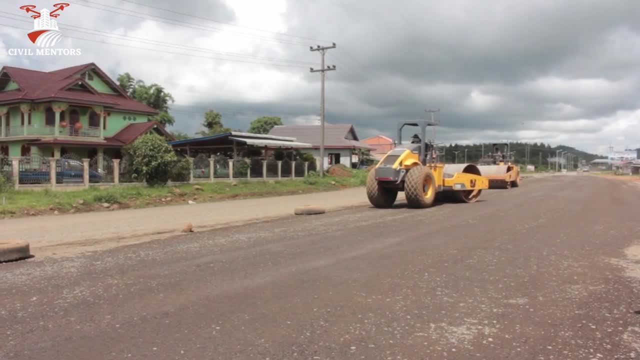 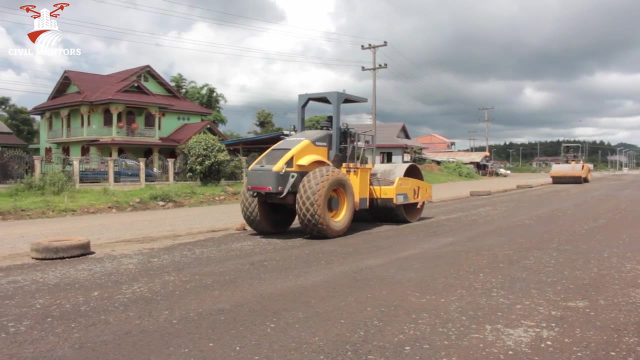 The base and sub-base layers provide support for the pavement and distribute the weight of vehicles evenly. The base layer is typically made of crushed stone or gravel, while the sub-base layer may be made of compacted soil or recycled materials such as crushed concrete or asphalt. This layer also helps to provide additional support and improves the 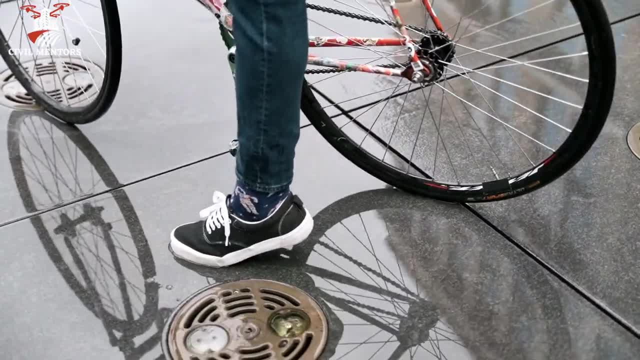 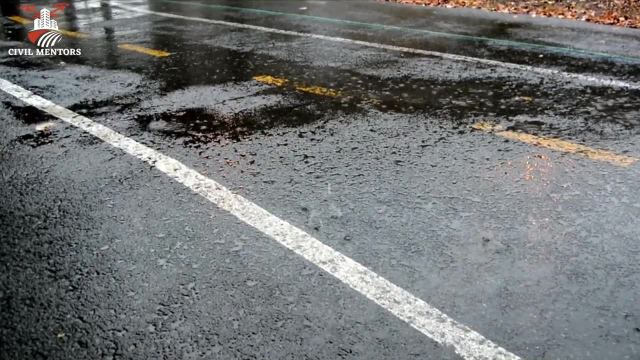 road's drainage system. Proper drainage is critical to the longevity of a road. The drainage system is designed to prevent water from accumulating on the road's surface and causing damage. This involves installing culverts, catch basins and drainage pipes along the sides of the road. 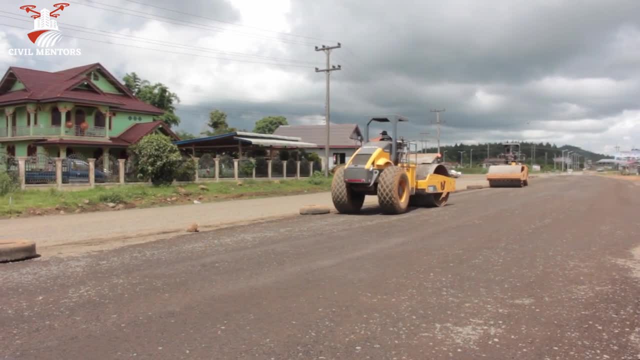 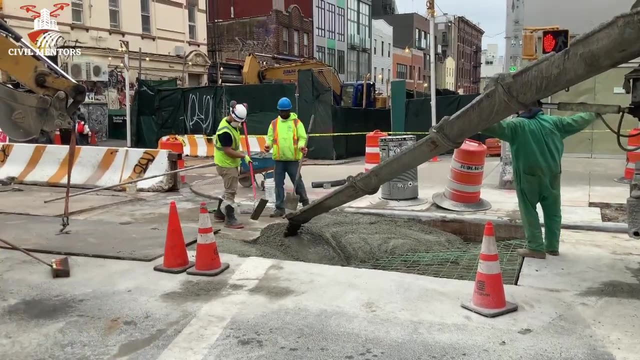 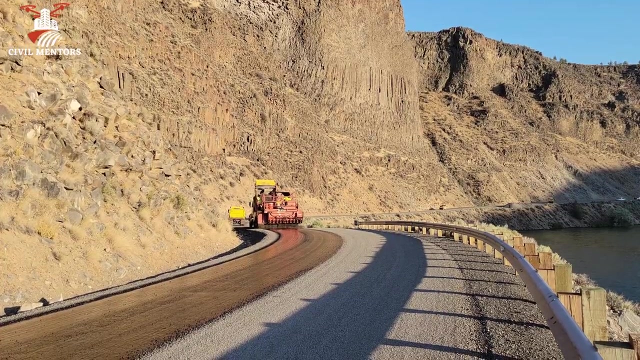 Once the base and sub-base layers are in place, it's time to pave the road. Asphalt is the most commonly used material for paving roads, although concrete may also be used for certain applications. The paving process involves laying the asphalt in layers and compacting it using heavy machinery such as bulldozer or roller. This helps to ensure that. 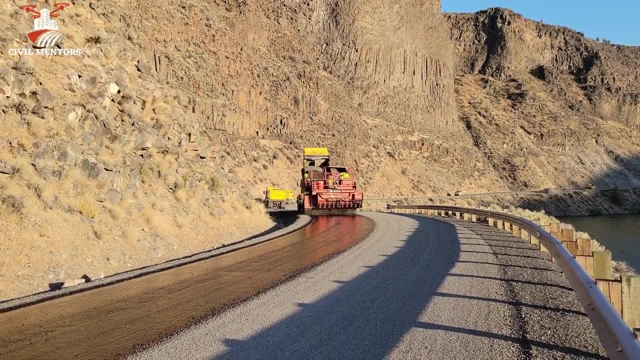 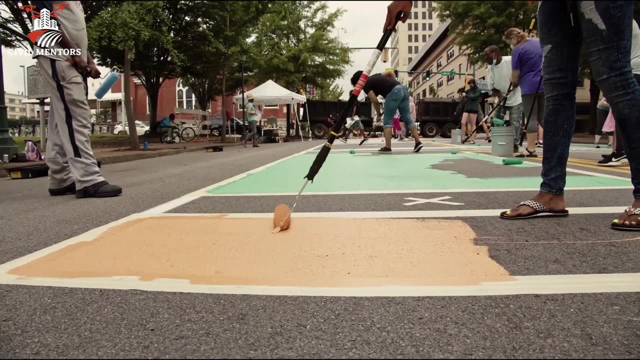 the pavement is smooth and free of air pockets, which can lead to cracks and other types of damage, And in some cases, the pavement is also used for pavement covering. With the pavement in place, the final step is to add road markings such as lane lines and symbols. 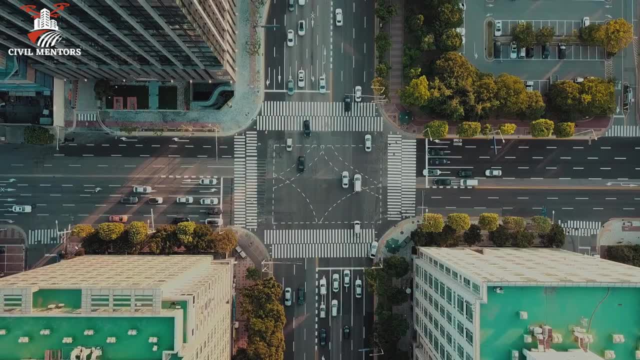 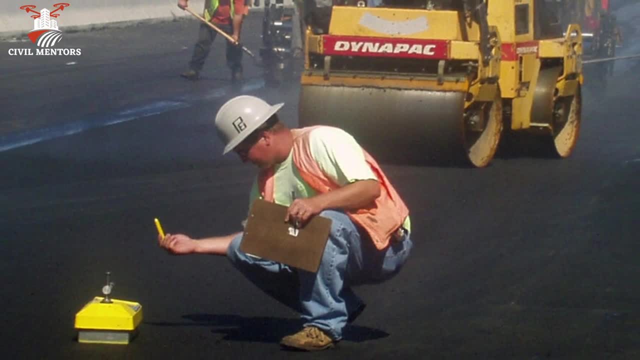 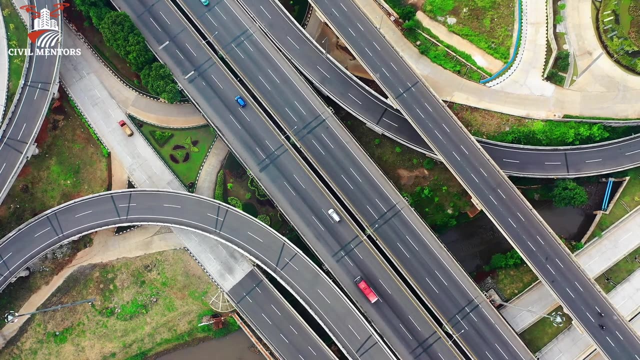 to guide motorists and improve safety. These markings are typically made using durable materials such as thermoplastic or epoxy paint. Once the road is completed, it undergoes a final inspection to ensure that it meets all safety and quality standards. If everything checks out, the road is opened up to the public and becomes an essential part of our 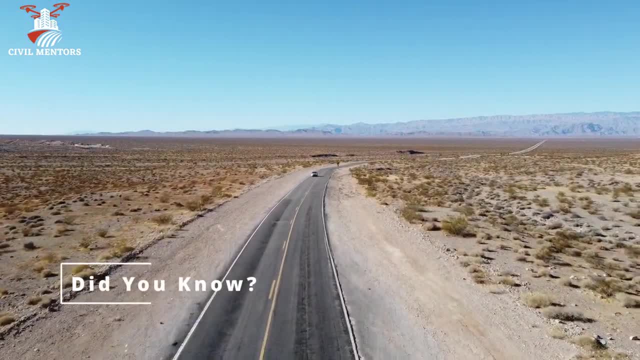 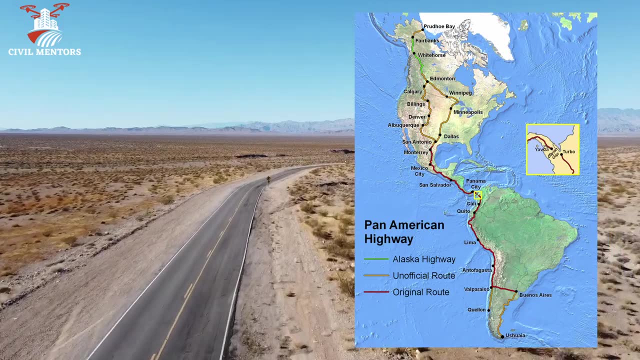 transportation infrastructure. Here is a fun fact. Did you know that the world's longest road is the Pan American Highway, which stretches from Prudhoe Bay, Alaska, to Ushuaia, Argentina, a distance of approximately 19,000 miles? 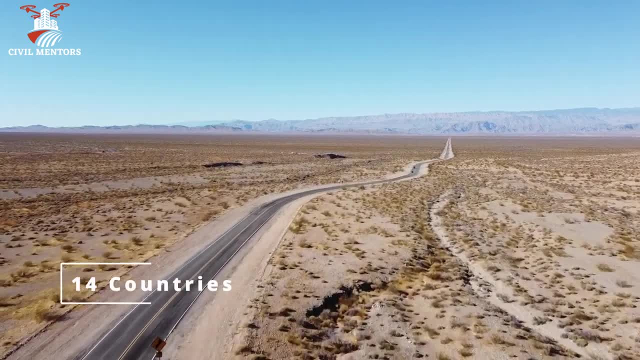 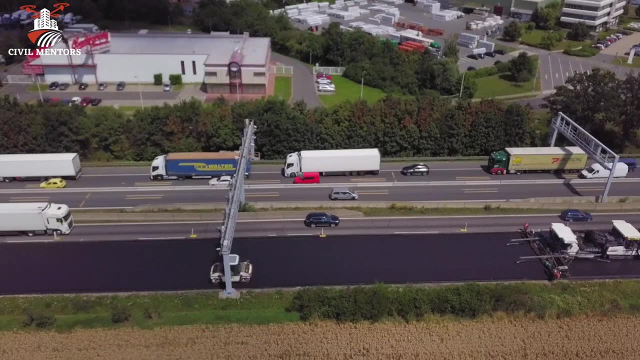 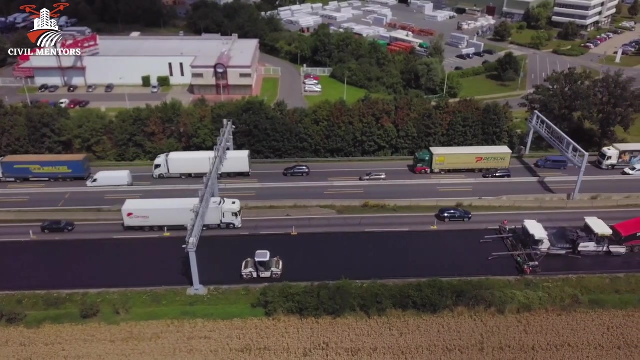 The highway passes through 14 countries and includes some of the most challenging terrain on the planet. Modern road construction is not just about asphalt and concrete. Engineers are constantly exploring new materials and technologies to create more sustainable and eco-friendly roads. For instance, some countries are experimenting. 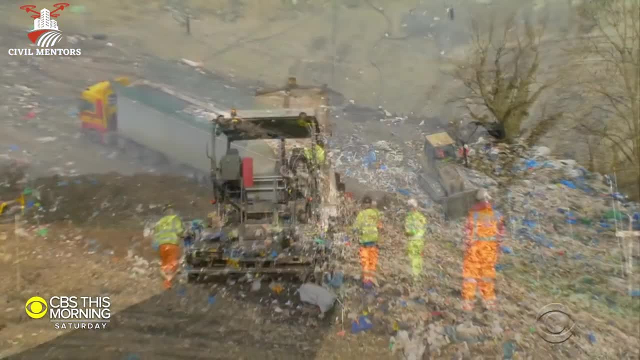 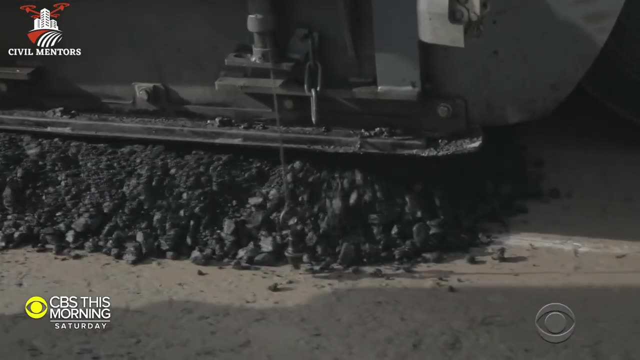 with using recycled plastic in road construction. The plastic is melted down and mixed with asphalt to create a durable and long-lasting road surface. This approach helps reduce plastic waste while creating a strong and resilient road. Another innovation is the use of geosynthetics. 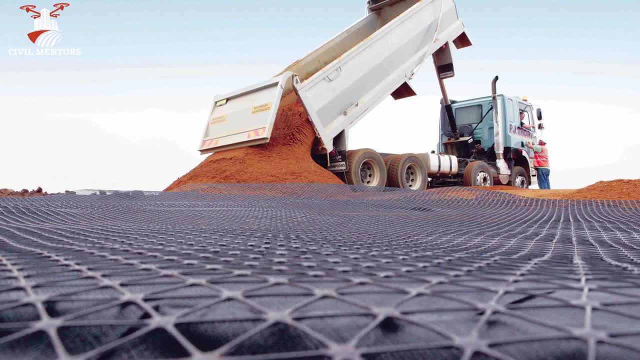 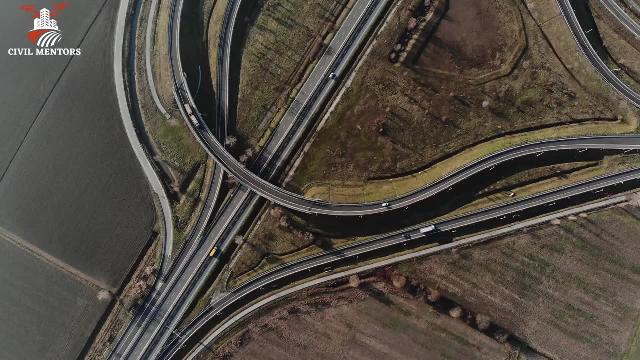 such as geotextiles and geomembranes, which can provide additional reinforcement and drainage for the road. These materials are cost-effective and can extend the road's lifespan. The construction of a road involves many different factors, such as the terrain, weather and traffic volume.